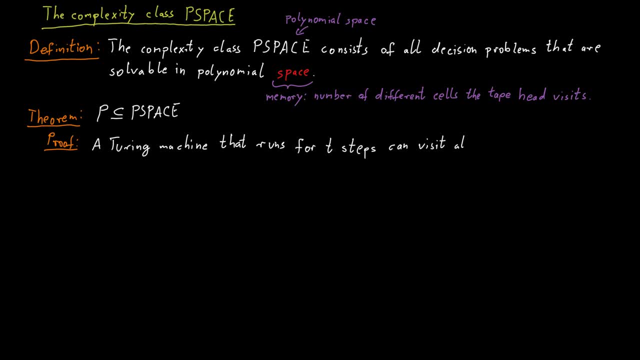 can also visit at most T different cells on the tape with its head. Restricting our computation to run in polynomial time is potentially more severe of a restriction than requiring the computation to run in polynomial space. The reason for this is that time cannot be reused, but space can. So if I have a certain 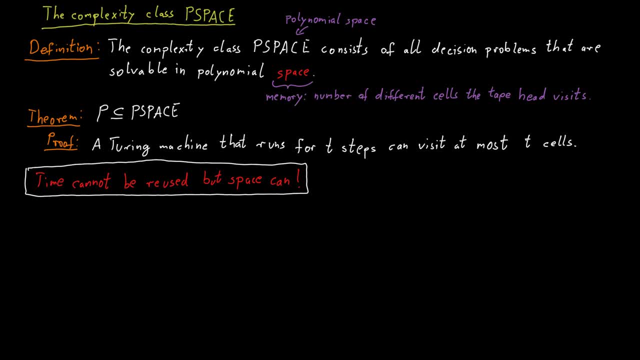 number of cells on the tape of the Turing machine that I can visit. then I can visit them again and again and store different things at different points in time, But I cannot go back in time and reuse time in the same way. I cannot go back in time and reuse time in the same way. 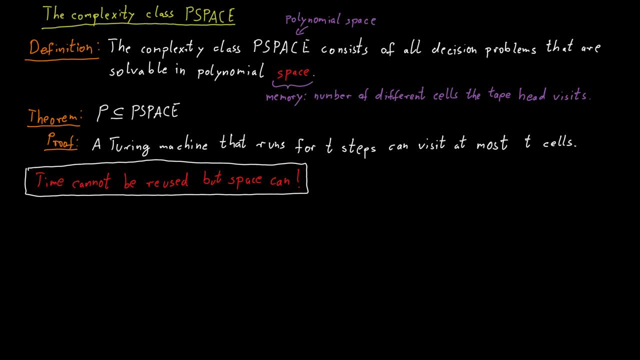 That is the relationship between time and space. But what about the relationship between p-space and np? As it turns out, satisfiability can be decided in polynomial space. We know that satisfiability is np-complete, so it is contained in the class np and belongs to. 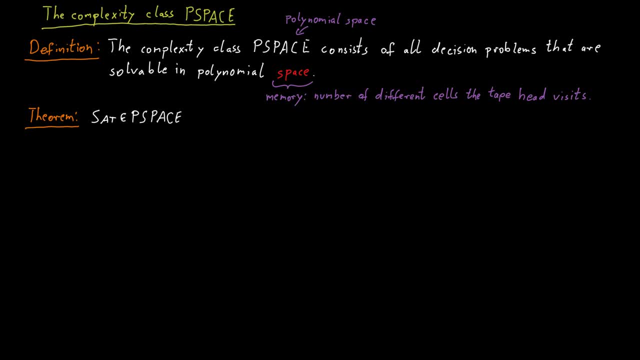 one of the most difficult problems in that class. Nevertheless, it can be decided in polynomial space quite easily. And here's how you do this. This is an algorithm for deciding satisfiability in polynomial space. We go through all possible assignments of truth values. 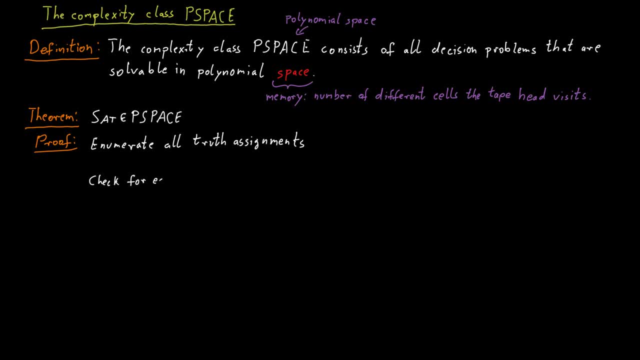 to the variables in the Boolean formula And for each possible assignment we check whether the formula is satisfied or not. As soon as we find an assignment that does satisfy the formula, we return true because clearly the formula is satisfiable. We found a truth assignment that. 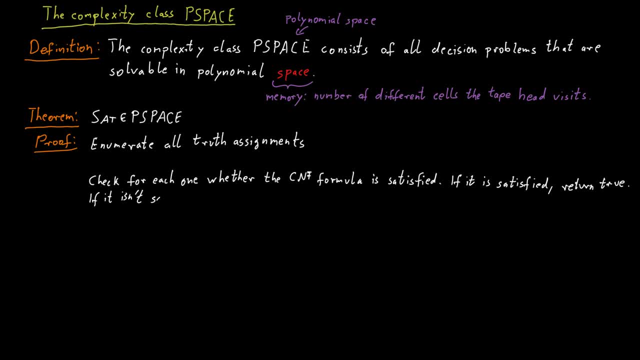 works. If, however, none of the possible assignments make the formula true, we return false. An implementation in detail. here is how we can enumerate all these assignments and plug them into the formula and test the formula, and so on. So here's how that works. We maintain a counter. 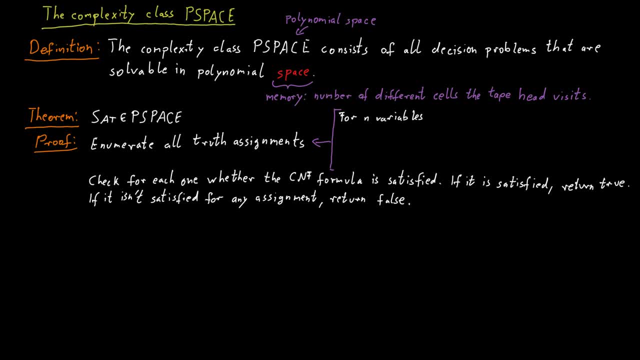 which is an n-bit odometer, where n is the number of variables in the Boolean formula. We start counting at 0, so we set all the variables to false And then, one by one, we increase the counter, which gives us a new truth assignment every single time. So, for example, let's say n is equal to 3, so we would: 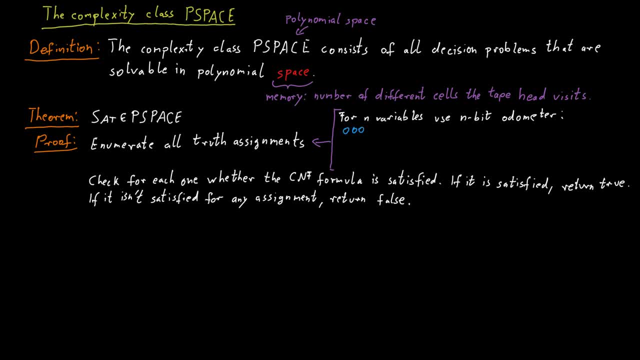 start with 000,, which means we set all three variables to false, And then we increase the counter, which would get to 001, so we would set the first two variables to false and the third variable to true, And then the next assignment would be 010, so the second variable would be true and the other two. 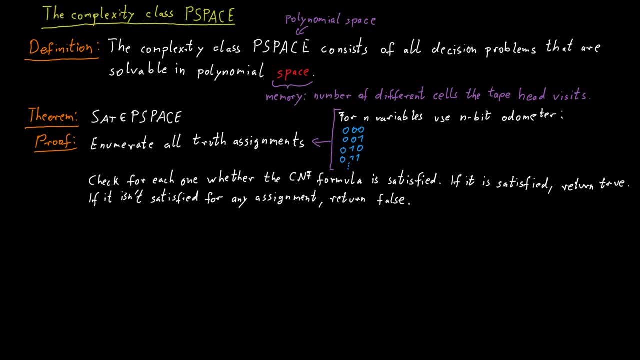 would be false, and so on. So in this way we can systematically enumerate all possible truth assignments through the n variables And for each of these we plug the values into the formula and evaluate the formula. Now, values for the variables into the formula and evaluating a. 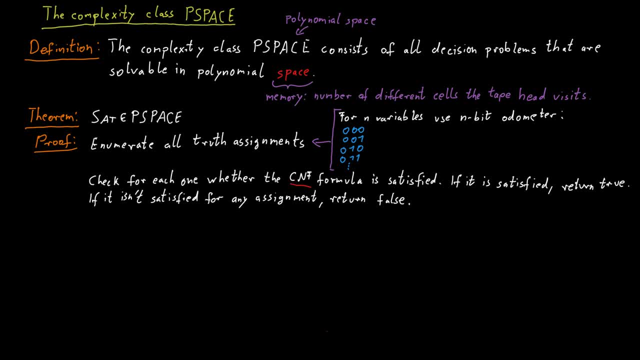 Boolean formula takes polynomial time, So each of those checks can be done in polynomial time. Since they can be done in polynomial time, they can also be done in polynomial space using the same algorithm And our odometer. as the name says, it's an n-bit odometer, so it only requires a polynomial. 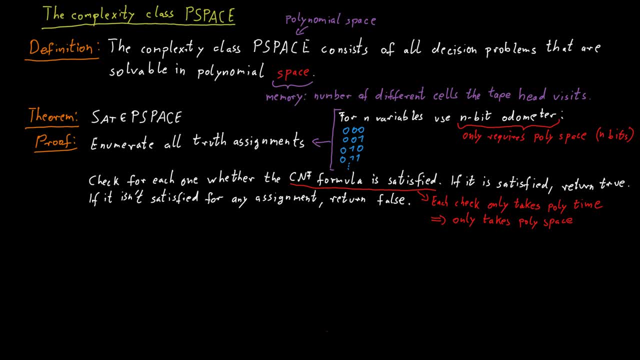 amount of space. It requires n bits, where n is the number of variables in the formula, which is polynomial in the size of the input, because the input needs to contain those n variables in some form. So the odometer can be maintained in polynomial space. 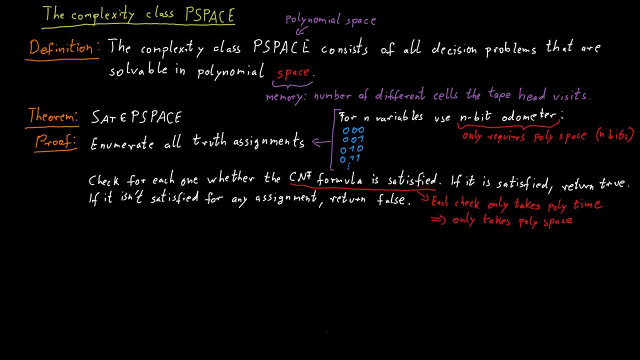 and each of the checks can be done in polynomial space as well. The crucial part here is that once we have checked a particular sort of odometer and we have done an assignment of variables, plugged this into the formula and evaluated the formula, we don't need to remember anything. 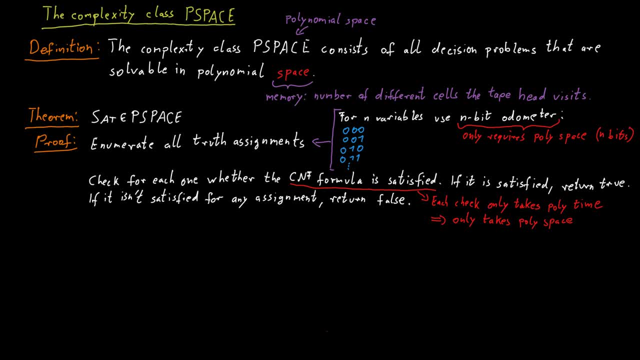 after that. So we can erase everything we needed to do to evaluate the formula from the memory and then reuse that memory for the next truth, assignment of the variables. And that is really the key here We can reuse this space. This algorithm requires exponential time because there are 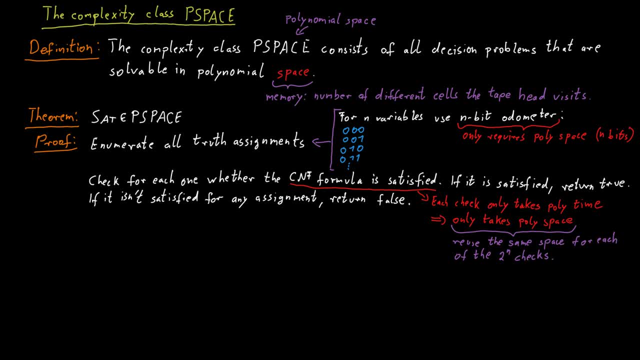 exponentially many truth assignments of the variables. But we only need polynomial space because we can reuse this space in each iteration of this loop of the algorithm, Since satisfiability is contained in P space and satisfiability is NP-complete, so belongs to the most difficult problems in NP. 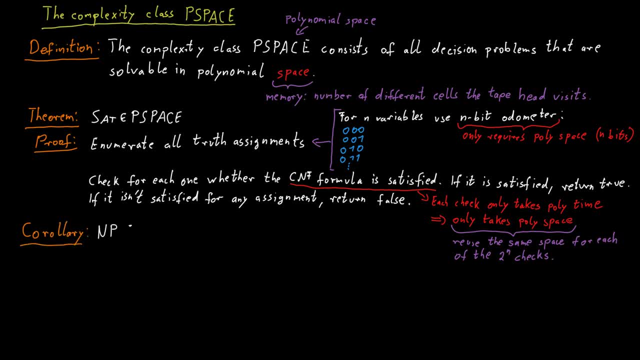 we should expect that all of NP is contained in P, And indeed this is true. The formal reasoning here is that if you consider an arbitrary problem Y in NP, then Y polynomial time carb reduces to satisfiability, because satisfiability is NP-complete, And so we can decide whether a word belongs to the language Y by. 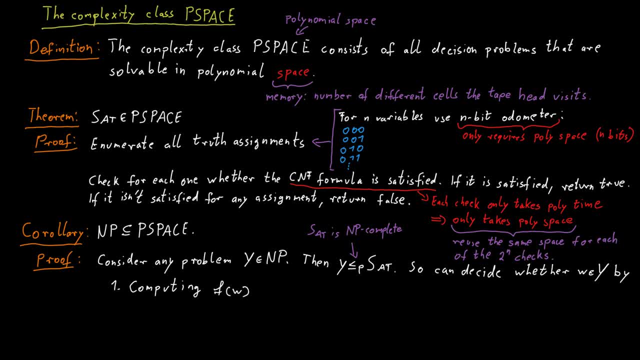 computing this function, this reduction function, this reduction F in polynomial time and then deciding whether F of that word is in the language satisfiability. As we have seen, we can decide whether a word is in this language satisfiability in polynomial space using this trick with the n-bit odometer. 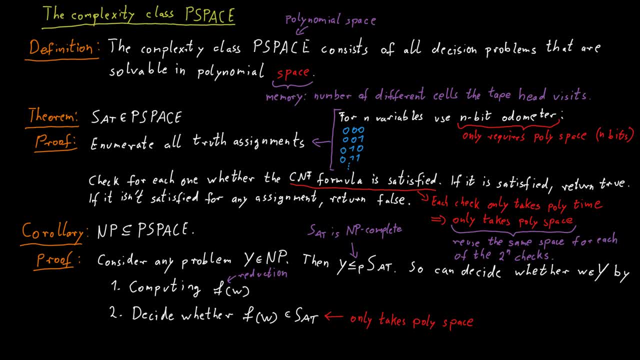 And so the second step of this process we can actually do in polynomial space, And the first step of the process we can even do in polynomial time. So clearly this also only takes polynomial space. So both steps in this process require polynomial space. So overall we can decide in polynomial space whether a word is. 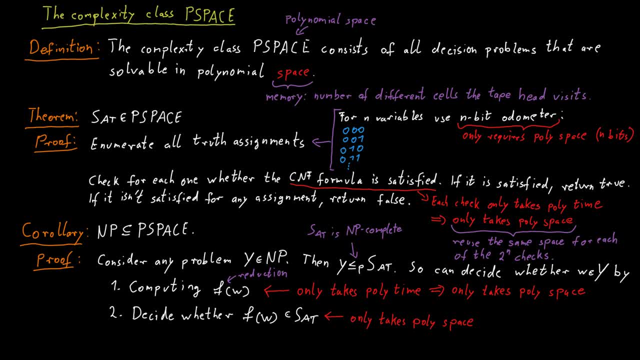 in the language Y or not, And therefore this language Y is also contained in P space. This works for any language Y in NP And therefore NP is completely contained in P space. There's a more abstract argument on why NP is contained in P space. 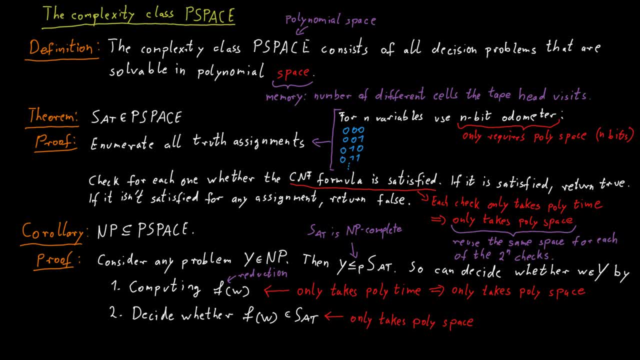 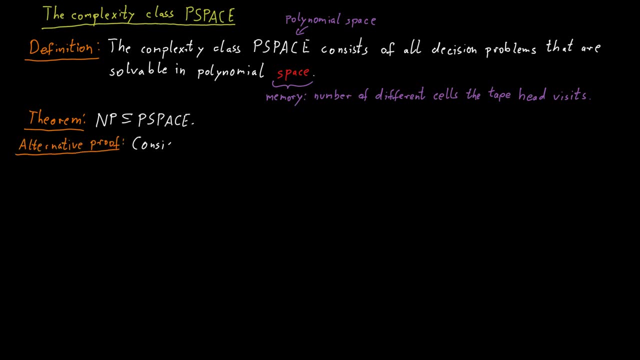 It sort of follows a similar line of thinking, but rather than using a specific problem like satisfiability for this argument, we use the definition of NP itself. So NP is the class of decision problems for which we have certificates and efficient verifiers, And these 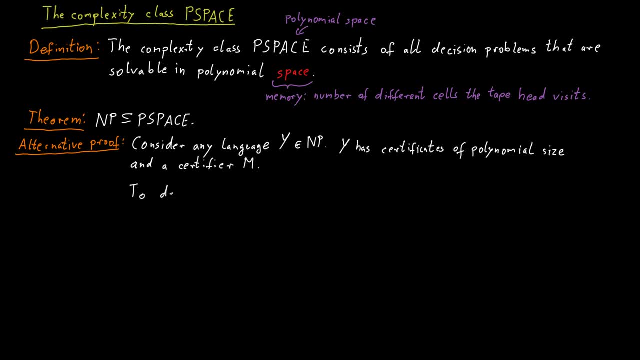 certificates have polynomial length. Therefore, what we can do to decide whether a word is in the language or not is to use this odometer to enumerate all possible potential certificates And then, for each of them, use the polynomial time verifier to check whether this certificate indeed certifies that the word is in the language. Y.